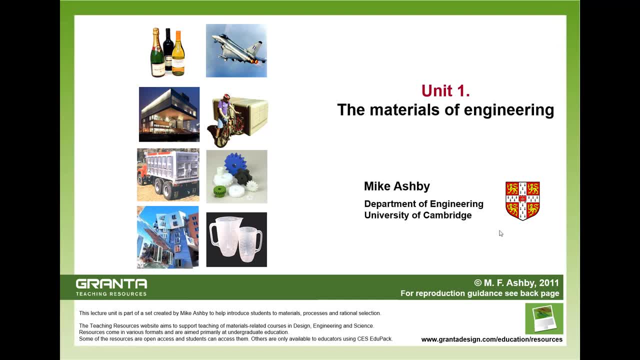 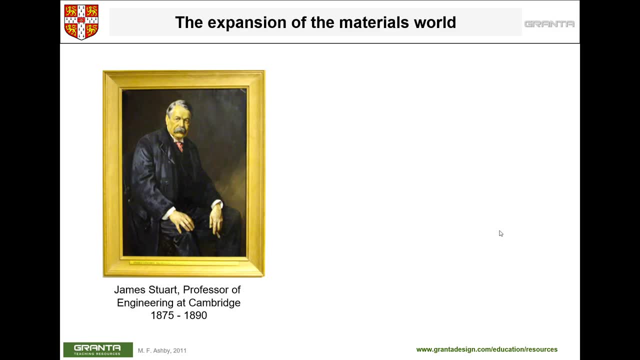 Hello everyone. Today we are going to talk about material selection, So material selection is an important part of the design process. As an engineer, after we have our design, we need to choose the right material for our design. James Stewart was the first professor of. 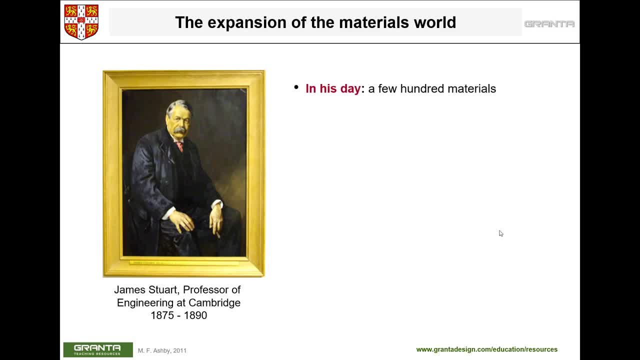 engineering at Cambridge University. At his time there were only a few hundred materials. There were no polymers or there were no synthetic polymers. Now we have thousands of polymers and or at least 45,000 known polymers. There were no light alloys, aluminum alloys and now we have. 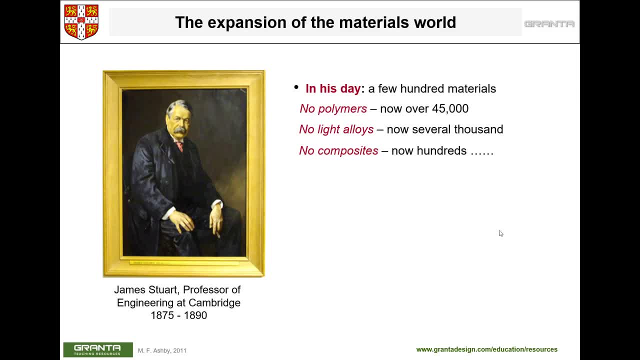 several thousands of alloys, And there were no composites or man-made composites. but now we can theoretically make infinite number of composite materials by combining different material categories, So now we have access to hundreds thousands of material, While this gives us the advantage of 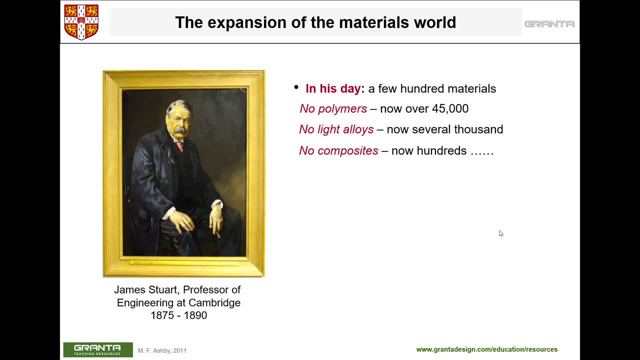 choosing the right material, but also it's very overwhelming. It raises the question how to choose the right material out of that many menu of selections. So here we are going to use Ashby Diagram or CES software to categorize materials and choose the one that works for our application, based on our engineering needs. 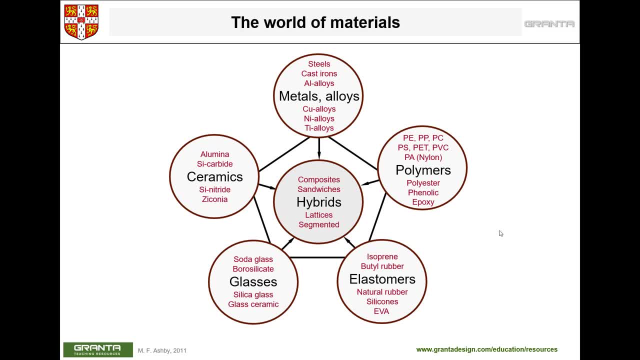 We can categorize material into three main categories. I mean sometimes it's grouped into five or six categories, but generally we have metals, polymers, ceramics and the combination of them which we call it hybrid. Glasses are usually grouped under ceramics, elastomers are. 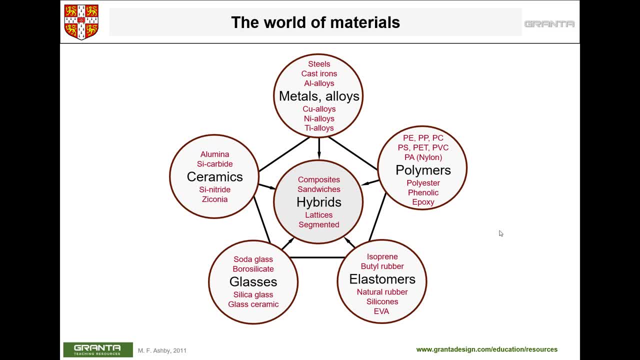 polymers and then plastomers are polymers that can stretch multiple times of their original size. So the strength to failure for our elastomers are few hundred percent. Remember, for the metals, the ductile metals, the strength to failure is only 5%. Water ladles have the advantage to stretch. few times their original length and they対向開廳根液が Alorselyенсelares object. you put them in and stretch and their policy is the same, Whereas a Oz Light Elastomer can stretch. several times the original length. seen here are a lot of metals. then I have some that I really like, but there is nowhere and a lot of José Bosque, Leslie, Doctor Congeř for doing those month or month, and we have allorisoulda determination. there's the advantage to stretch the lasts over time, the original size And they are. 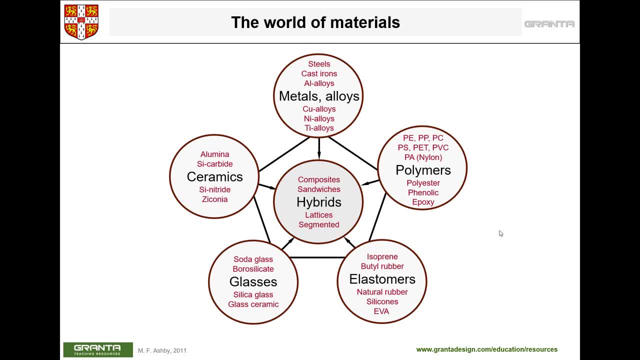 have their own application in different industries. Whenever I think of metals, whenever I want to use metals, whenever we need high strengths, high modulus or high conductivity, metals are our first choices. And within metals we can use steel, cast iron, aluminum and so forth. But they come with a disadvantage: They are 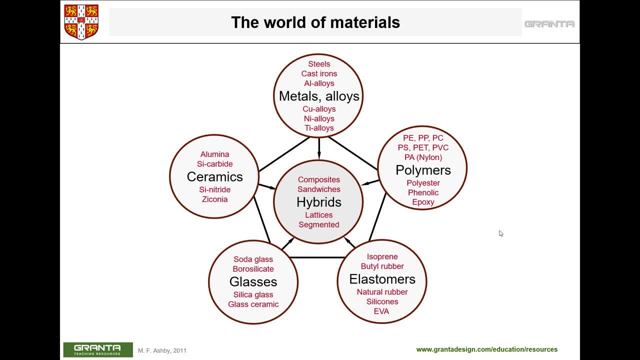 very heavy, And when the weight is an issue, you might look into other options. The manufacturing of metal is not as easy as polymers. The cost of using metal is not desirable either When we move to ceramics. when high temperature is required- resistance to high temperatures- ceramics should be our number one. 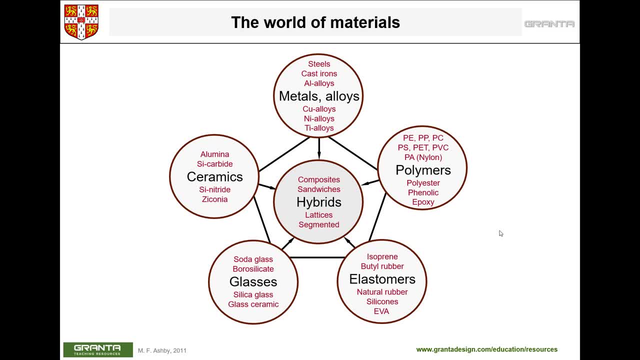 choice. They have a very good temperature resistance. So in a sports car, whenever you have the ceramic, you have ceramic brakes because they can handle high temperature. In aerospace applications, when a shuttle enters the Earth's atmosphere it undergoes a very high temperature gradient and the 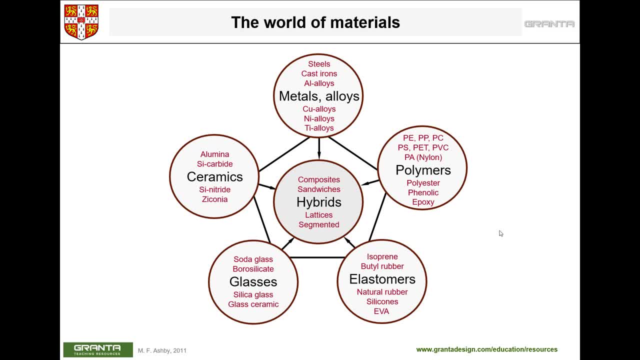 outer surface is made of ceramic alloys or ceramic composites. But again, there is always a trade-off. The trade-off with ceramics is that they are very brittle, So they don't have any ductility And the manufacturing process is challenging. So, as a designer, you need to look at the 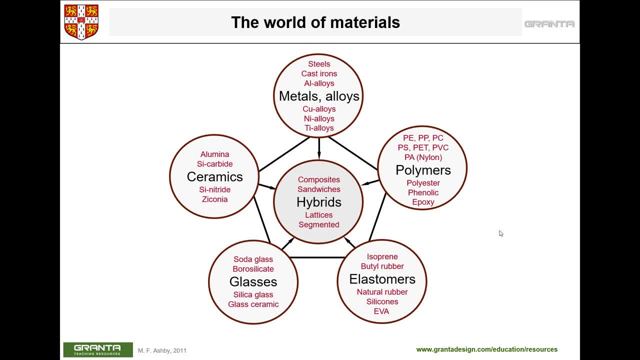 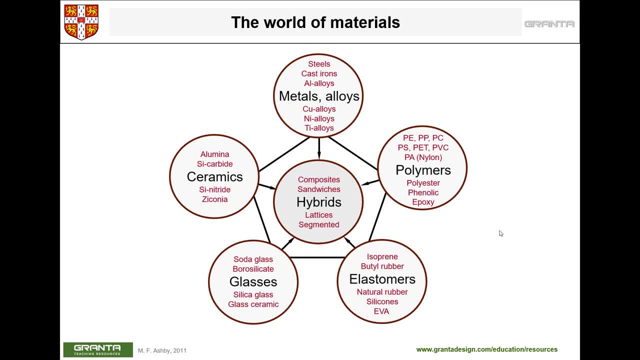 and keep their advantages and offset their weaknesses. so we said that polymers are very light but they're not strong. so what if we add, let's say, carbon fiber to polymer, so we can keep the light advantage of the polymer and offset the weakness, which is which was the strength? so now we have a carbon 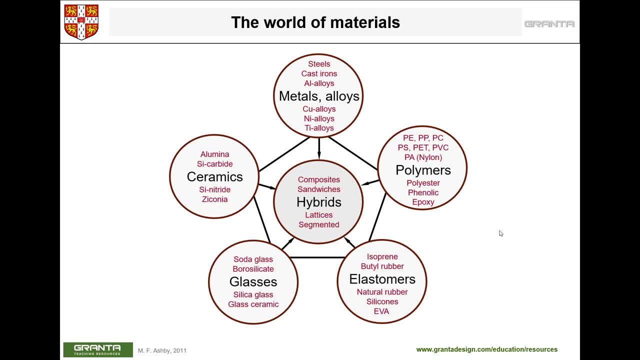 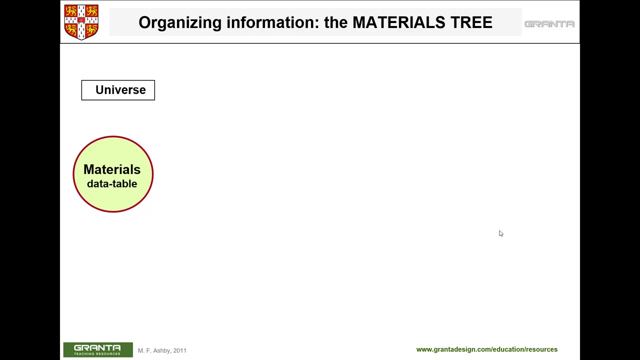 fiber reinforced polymer which is both strong and light, and that's when composite comes into play. so we tailor the material to our applications. we put this transfer, we want it so, not only designed with the material, but designing the material itself in your design process. first you have different. 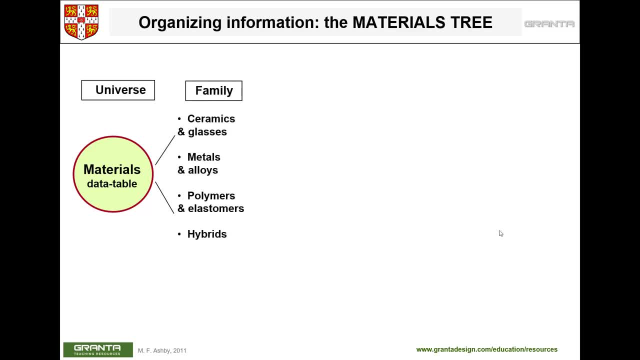 you need to think of the big category of material, the family that you are dealing with. are you going to go through ceramic metals, polymers or polymers- if you are going to go through power and energy or whatever those are, composites- and once you selected your category, saying that, okay, I want to go with metal for my 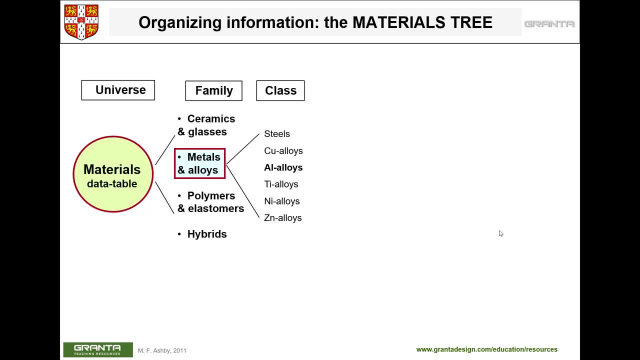 application metal would be the right choice. then you could go to the subcategories: are you going to use steel, are you going to use aluminum, titanium and so on? and then, if you choose aluminum, we have a different range of aluminums and different alloys. you can narrow it down to. 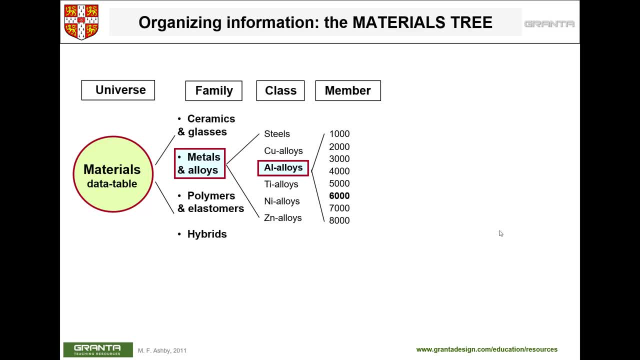 aluminum 6000, and once you selected that material you can go and check the material properties, the density, mechanical properties, thermal, electrical, optical properties and to see if it fits your application. these properties that clearly give us a value. we call it structured information. and then there are some information that we do not have any quantity for them but are very helpful in. 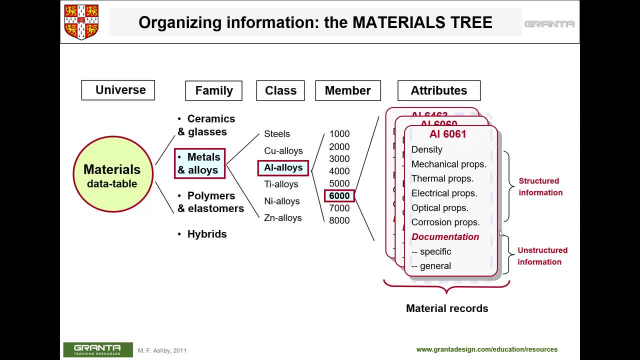 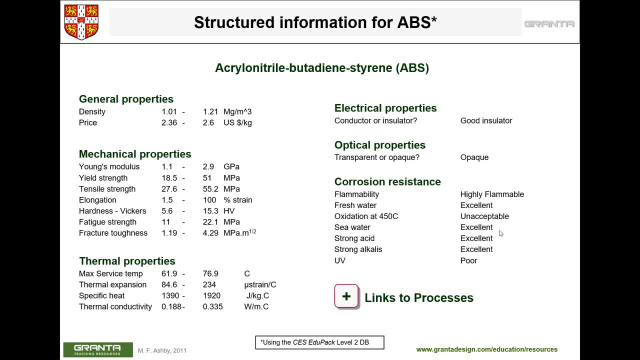 the application process in our design, and then we refer to do them on a structured information. so here I'm showing you an example of structured information for a polymer ABS. it gives you the general properties, densities, the price per kilogram and then the mechanical properties, which are Young's modulus yield. 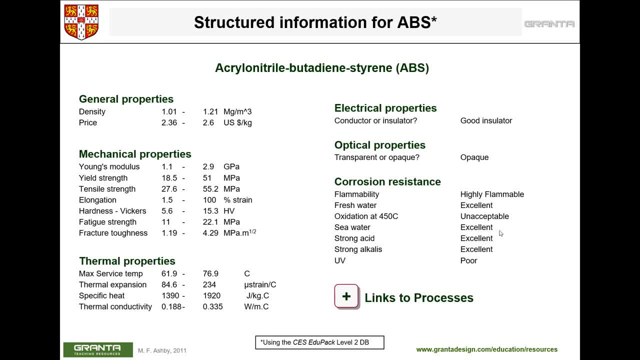 strengths- tensile strengths, elongation, hardness, fatigue, fracture- and, depending on your application, one property might be important and another. as you can see, there is a range of properties, because each time we break a sample, we test the sample, we are going to get a different result, so there's always a variability, so you can. 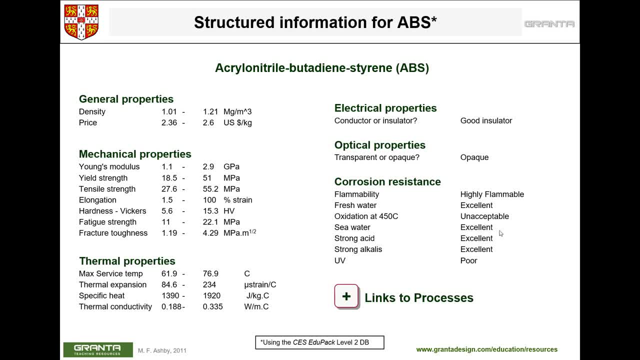 either take an average of these two numbers that you see here. there is a range from 1.1 to 2.9 giga Pascal. you take an average or use, but also, in addition to the average, you need to pay attention to the variability. if there is a large variability in a material property, that means that there is a 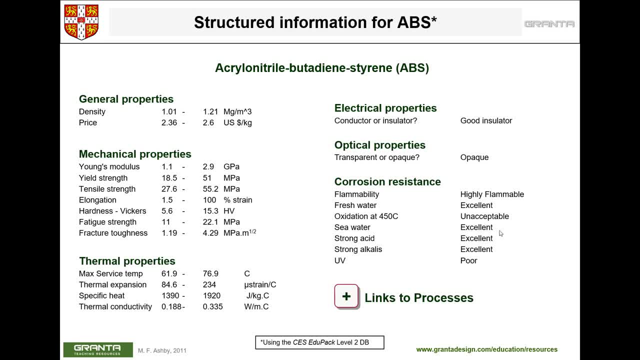 low reliability. so, depending on your application and the reliability that you want to use, you might use the lower number to be safer. and again, in mechanical engineering, everything is application dependent. whether you are designing an airplane or a bicycle, your design procedure would be different, your reliability level would be different. and here you can see on the right: 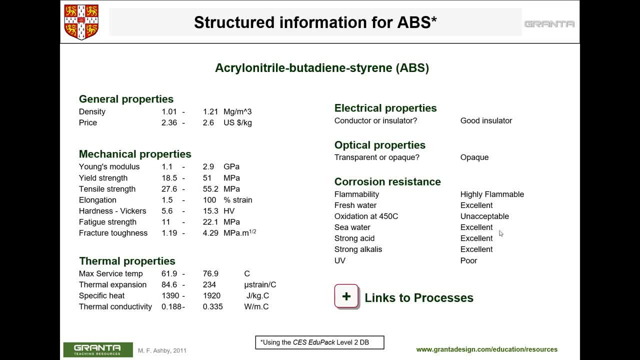 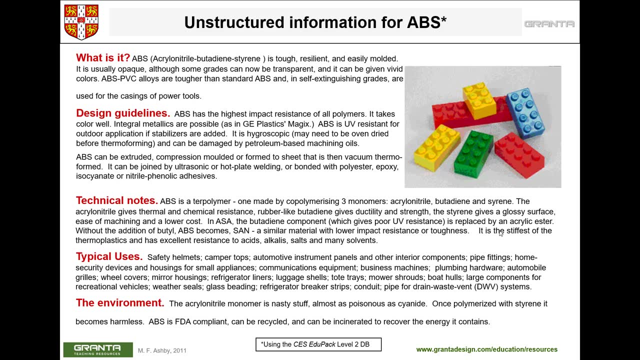 side, you can see other properties such as electrical properties, optical properties that are associated with a specific number- what, but it indicates that are a good conductor or insulator. and here is a honest structure, information that gives you information about the material and design process, and some notes to give you some insight of how to use the material in different application. 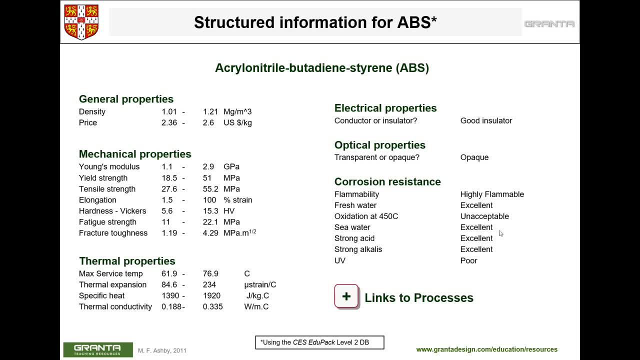 and if you look at here at the bottom you have a links to process. so this is, this is the information you have in the CES software. so you could, in a CES software for any material that you are looking up, you can link to process to see what processes can you use to manufacture this material. can you use? 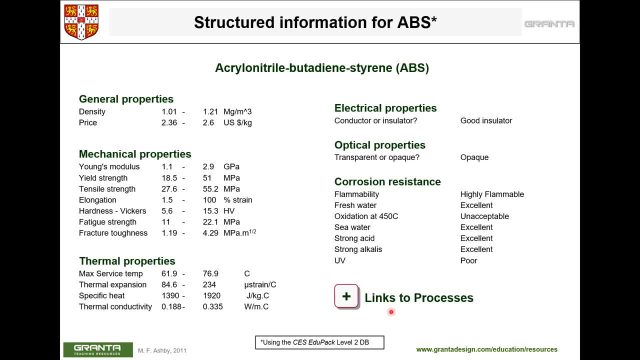 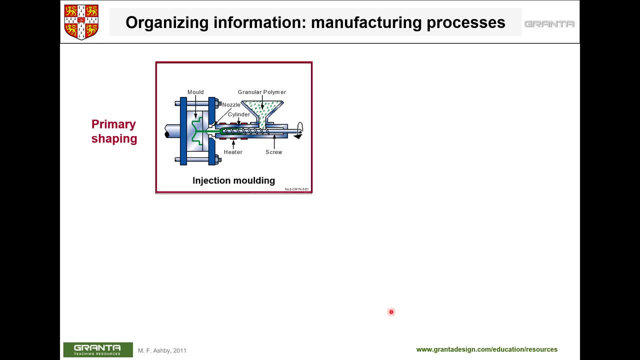 injection molding, compression molding, casting, additive manufacturing and so on. so it links process to material properties. for processes we have four main categories. we have primary shaping, which would be injection molding, compression molding, 3d printing, and then you have the secondary shaping. well, if you have your material, then you could use machining like late milling. 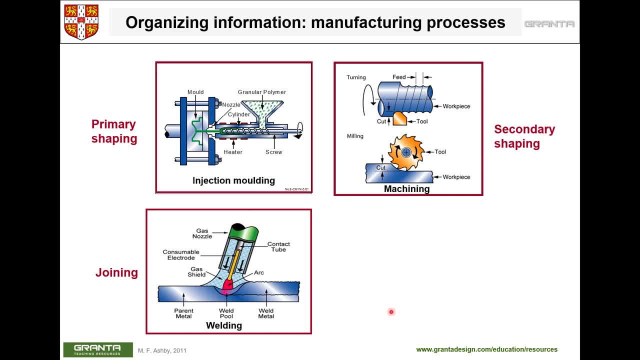 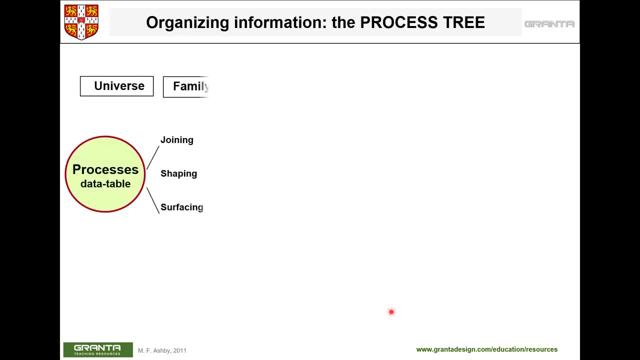 and machine your part to your desired geometry, and then you have the joining. if you want to join two materials, and the last one would be the surface treating, whether it's painting, coding, polishing, that would be the last process of your process tree, so similar to the material process. for, for manufacturing, you have the family. 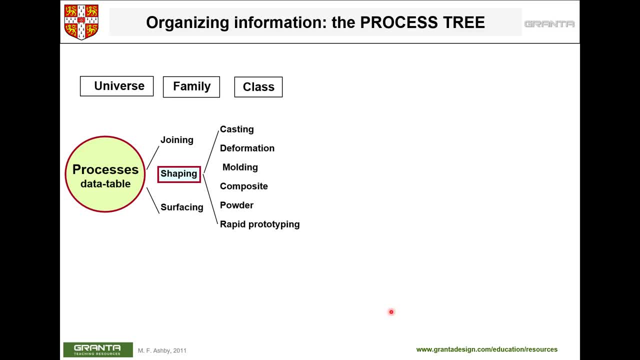 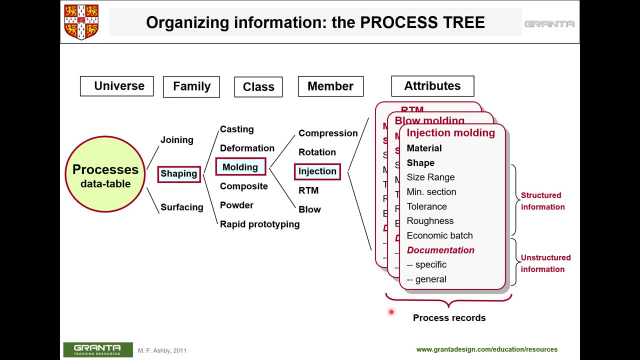 category which would be joining shaping surfacing. if you are choosing shaping, you could use molding. in terms of molding, you have different types of molding: compression, rotation, injection- and if you choose the injection in the software, it gives you a range of value and processes that you could apply to the size range, the tolerances that you're going to. 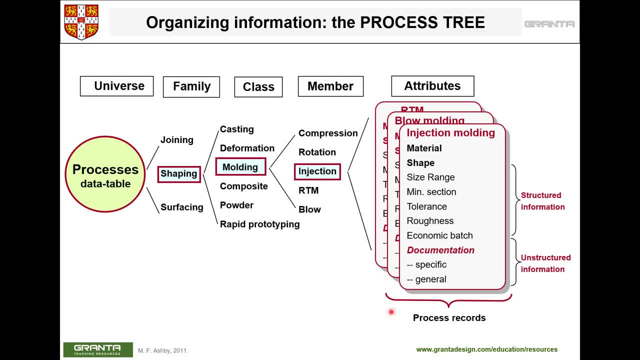 use the roughness. so reading those information will give you insight whether that process is suitable for the material that you selected, because not only we have to select the material, but we have to manufacture that material to our geometry. if your geometry is so complicated, maybe the only option that you have is 3d printing. 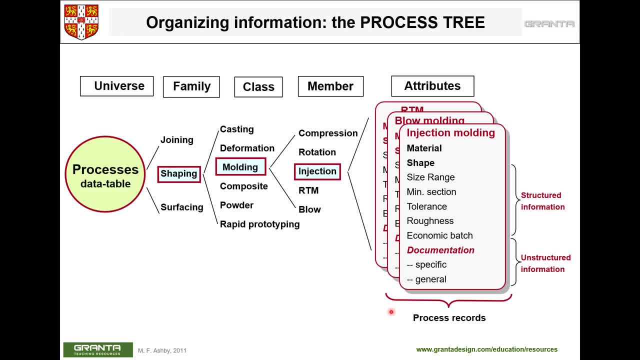 but also it's very expensive if you're dealing with ceramic. 3d printing of ceramic is very expensive. so as an engineer, you should not solely look at one category. you have to keep in mind all different uh limitation and trade-off that you have and here in manufacturing process you have. 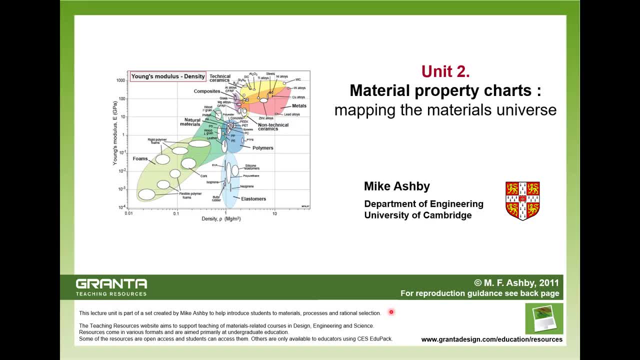 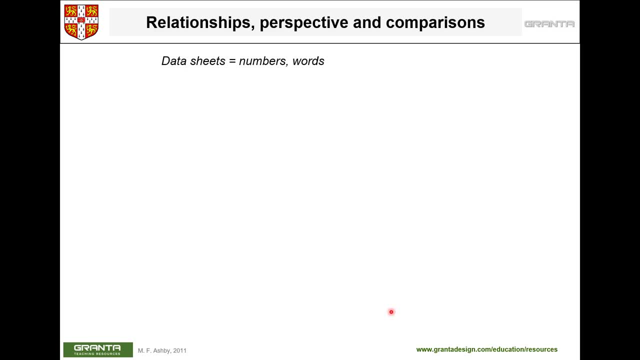 structured information and unstructured information, but we want to compare material together because that's true that we have. we can have access to different data sheets, but those give us numbers and words and we want meaning. we want the material property chart to compare out of these thousands of. 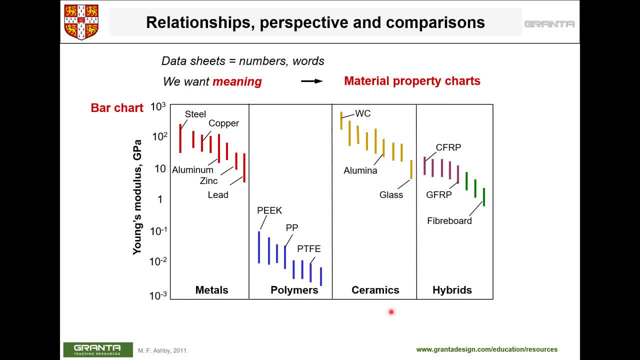 material with different properties, which one is suitable for us? so the best way is to plot them. so here i'm showing you a plot of young's modulus for different material. so it's just uh y-axis here. it's based on gigapascal. you can see metals, polymers, ceramics. 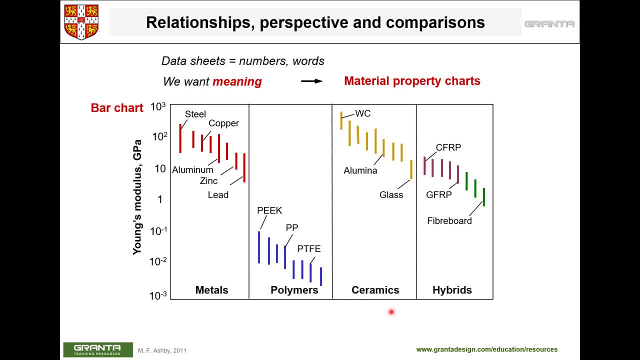 and hybrids. you can see metals of course have a higher young's modulus and polymers have a lower young's modulus. here because when we are comparing material from different category, from polymers and elastomers to ceramics and metals, we are dealing with a long range of property. we use logarithmic. 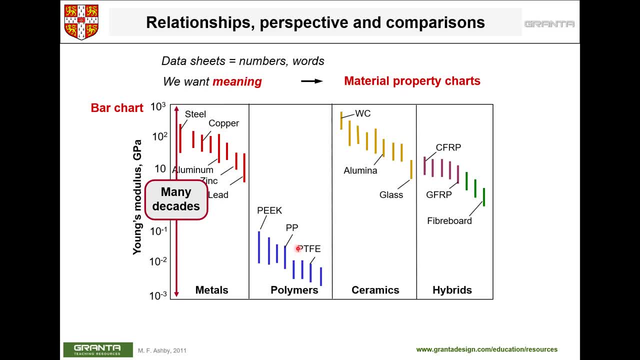 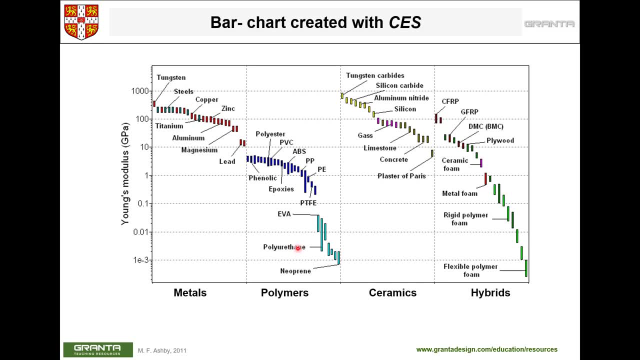 so you can see the y-axis is as many decades is in a logarithmic scale, we can cover a longer range and here it shows the same plot but with more information. we have opened up the groups of material so you could compare, if you are, if you. 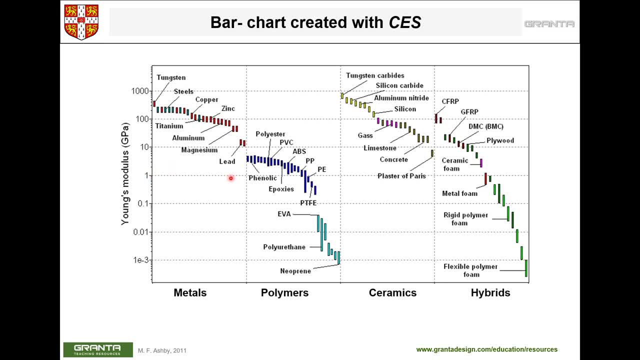 want a material with Young's modulus more than one, then you have to select the material on top of this line and you could plot these figures in in CES software. if you want material with high modulus, that's the group of material that we need to deal with. if you want material with low modulus, of course you. 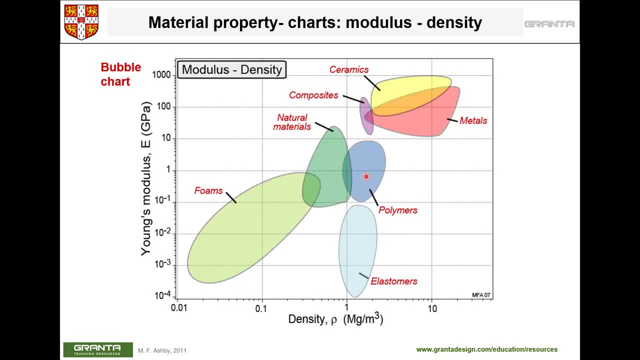 have to select the bottom part of the plot. but to better displace the material, we need to plot Young's modulus as a function of density or weight. we want to have a function of density or weight. we want to have a function of density or weight. we want to have a function of density or weight. we want. 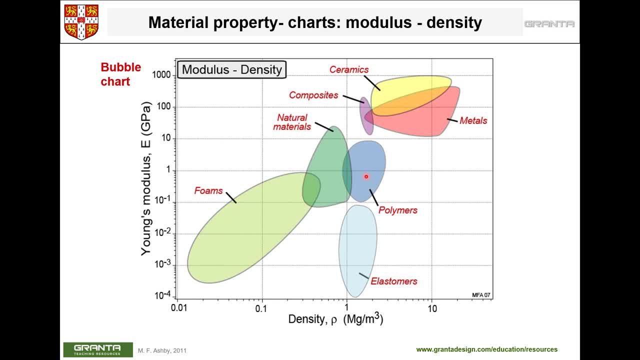 high strength per weight. so composites might not stand well when you compare it with young modules of steel. but when you plot as function of weight you can see composites are comparable with metals and ceramics because they all have high strengths and also they have lower weight and then polymers won't be a 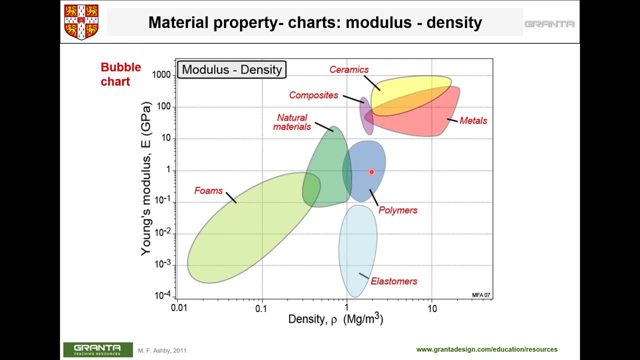 terrible choice either, because that's true that their modulus is not that high, but the density is is pretty low. so plotting y against X for different property, looking at two properties at the same time, would be very helpful for us Here. we're just interested in the modulus and the density of the material similar to other. 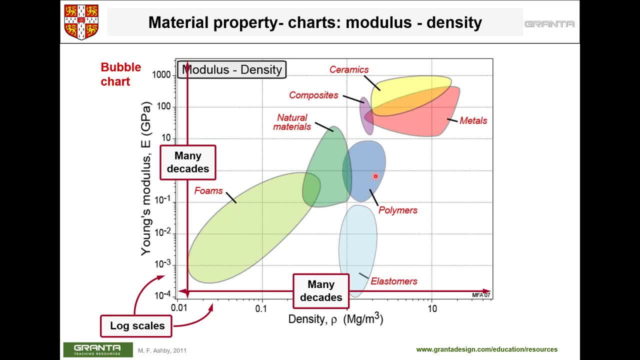 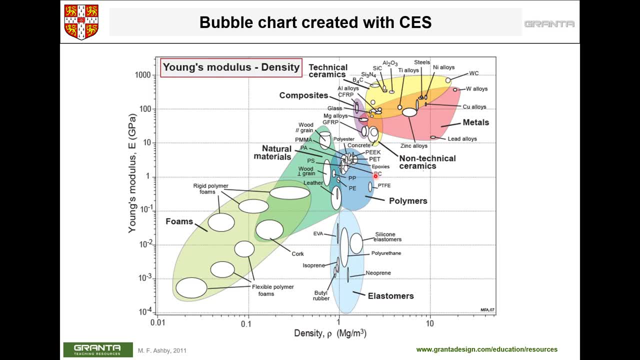 plots because you're dealing with a long range of material. we are using logarithmic scale. here is the same plot, but we have clicked on each category to come up with the material that that it encompasses. you wants to select the upper right here: high, young, modulus and high density. here you can select a line which would be, let's say, 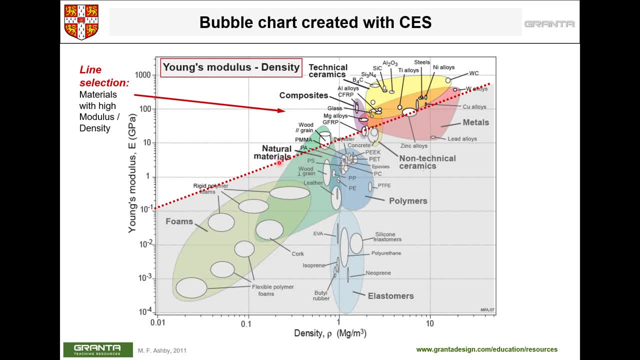 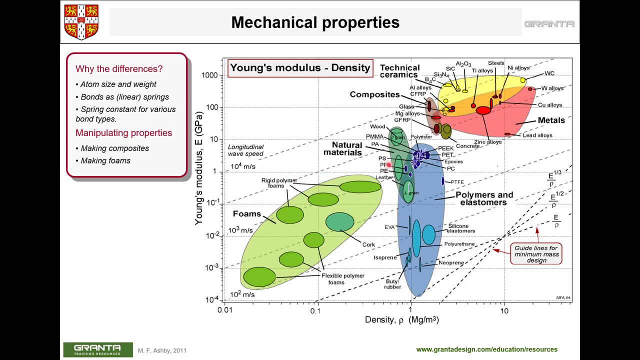 if the linear is logarithmic. so you want to select the young modulus per density higher than a specific value, so you have to select all the material. that's all on top of this line. and here is the same plot but the different lines and you can see the equations of each line here. so here is e to the power of 1. 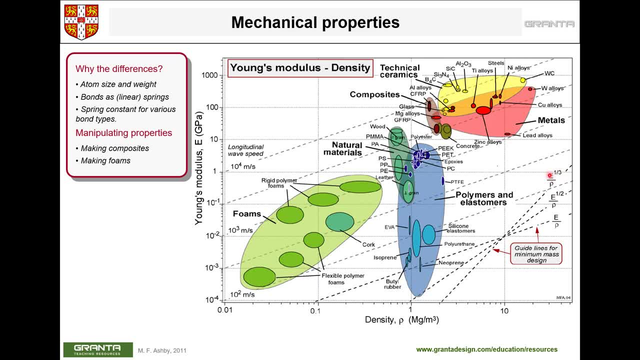 terrible. we are dealing with logarithmic scale, so this comes up as a linear line and, depending on your design choice, you might deal with different lines. if you are only interested in elastic modulus as function of the density, okay, that's. that's the line that you deal with. 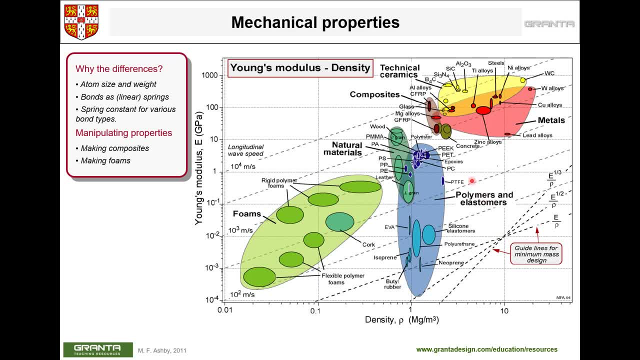 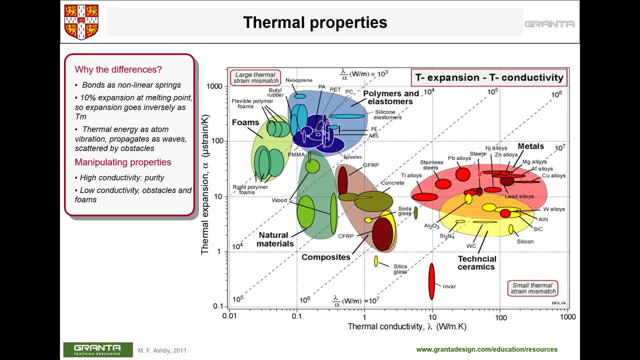 and if you want it to be higher than a specific value. this line is moving up and down to meet your criteria. similar to the mechanical properties, we can look at the thermal properties. the two common thermal properties that we are interested is thermal expansion. so when you're heating up the material, how much? 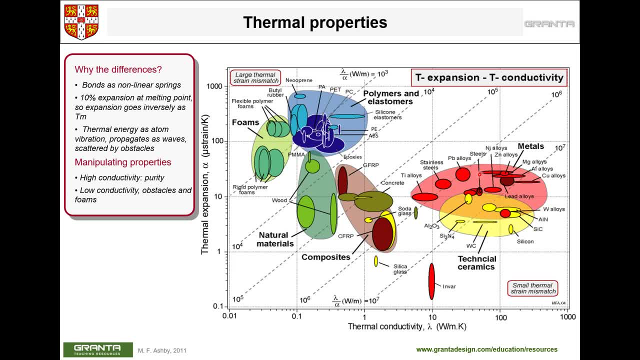 it shrinks or expands, and also thermal conductivity, when you're heating one corner of material, how it transfers to the other part of material and application. you want your material to be conductive or whether you want to be have a very low conductivity to be for your insulators. you want a lower conductivity for thermal. 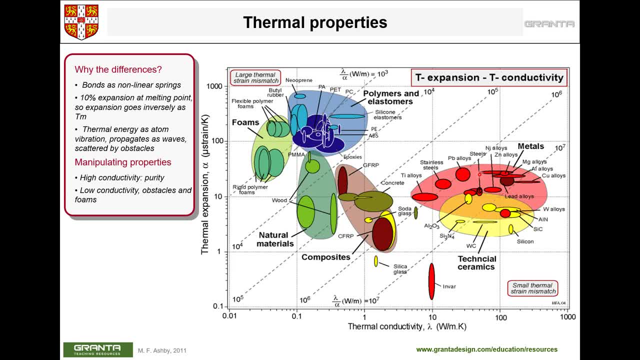 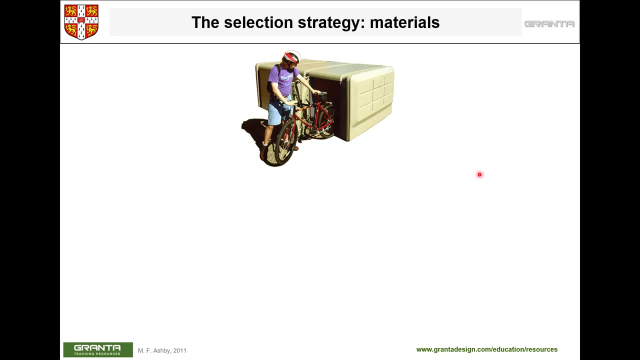 expansion for most application we want low thermal expansion. we don't want our material to to expand or shrink significantly with the change in temperature, unless you're designing an actuator which which functions on expansion and shrinking of the material. and here we are. you want to go through a selection process. let's say you're going to design a shed for your 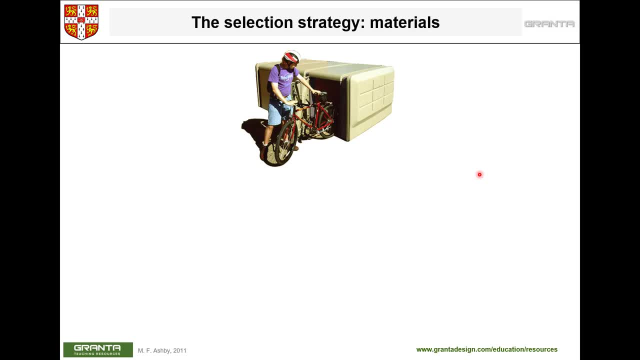 bicycle, so to cover it during winter. first you need to come up what are your design requirements. design requirements: we're going to list them as constraints and objective constraints, or the ones that we use pass and fail, theory that you, your design, must meet those constraints. objective: you: 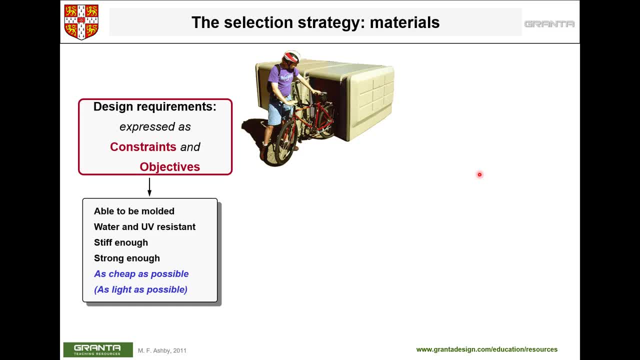 are going to minimize or maximize. so, for example, here your constraints. you want it to be able to be molded because you don't want it to be expensive. molding is is one of the cheapest manufacturing method. you want it to be water and UV resistance because you want to keep it outside. so it has to be with a stand. 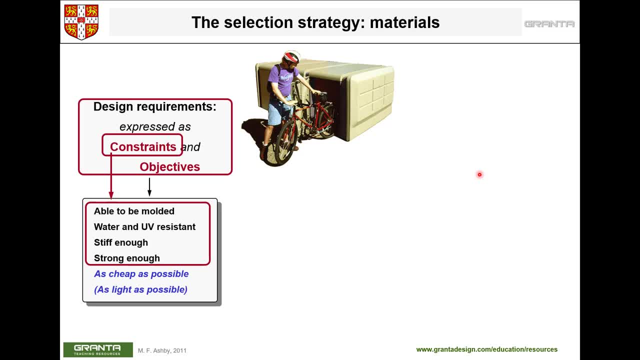 during winter. you want it to be stiff enough so it doesn't fail, it doesn't deform, and you want it to be a strong enough so it doesn't fail. but also you want it to be as cheap as possible. that's your objective. you want it to be as light as possible, that's your objective. you don't have. 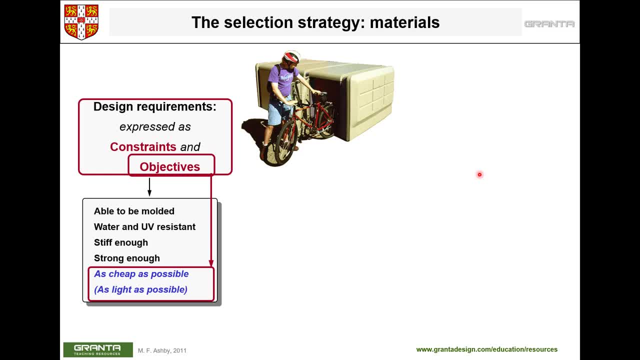 a specific value, but you want to minimize that. so that's an objective. but for molding and UV resistance is a constraint. if it doesn't meet those constraints it's not going to go through the next screening process. then you have your material, so you have your design requirements. on 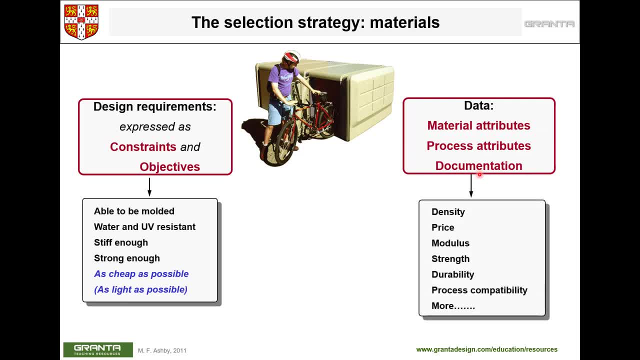 one side you have the material attributes, the process attribute on the other side, which gives you information about density, price, modulus, strength and durability. so you're gonna put all the material through the screening process to make sure that the and you're going to narrow it down to material that passes your constraints. 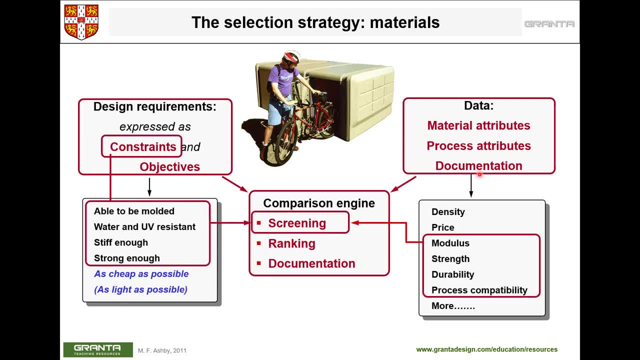 and that we call it screening. and then, once you screen and then get rid of the material that do not meet your constraints, then you're going to go through the rank. you're going to rank them based on price or you're going to rank them based on weight and select. 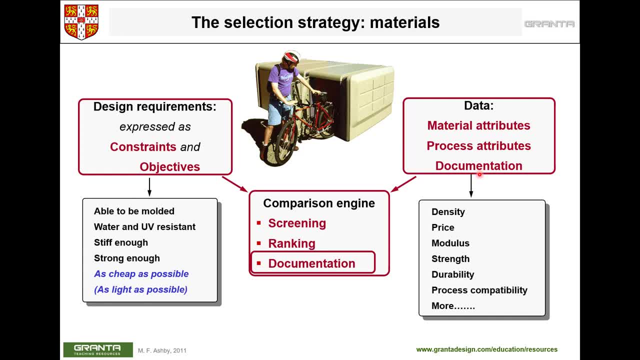 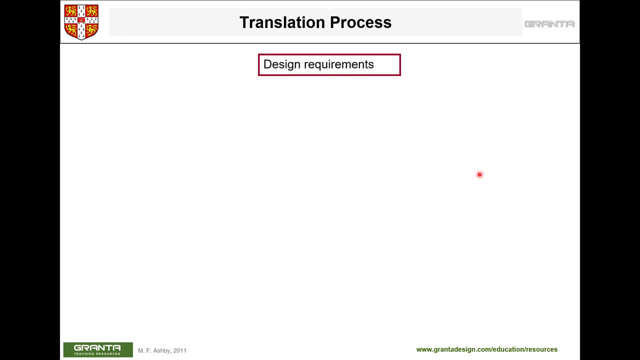 the best choice for you, and all of these are are are doable by CES software. you just pass it through a screening process and pass it through ranking and it ranks you the best material for your application and you will have your final answer. so for design requirements, you have function. you. 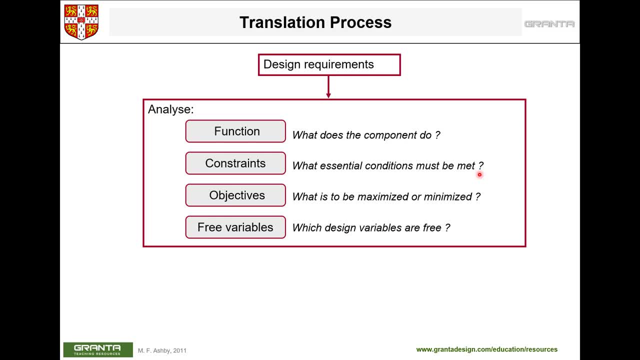 have constraints. what essential conditions your material well must be met. then you have objective. so for screening process and selection process, constraints are the one again that you have a specific value for it or you it has to meet an objective are the one that you want to minimize or maximize. you want to minimize the price. you want to minimize the weight, you want. 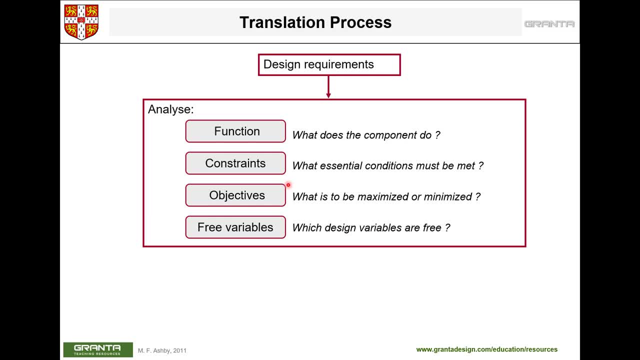 to maximize the strength, but you don't have a specific number for it. and then you need to know what three valuables you have, so you could use that free value but your or your performance index to find the right material for your choice. then these are all your translation and you have your. 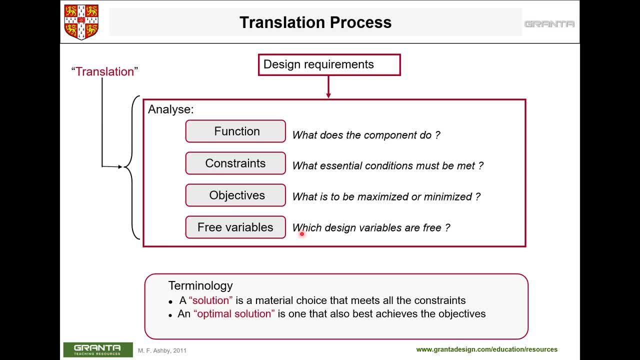 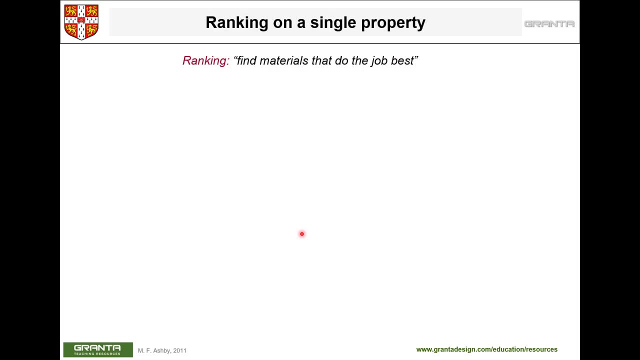 solution. so all the material that meets the constraint would be a solution, but the optimal solution would be the one that achieves the objective as well, the solution. you will get a solution through the screening and the get the optimal solution through ranking process. so let's look at a simple 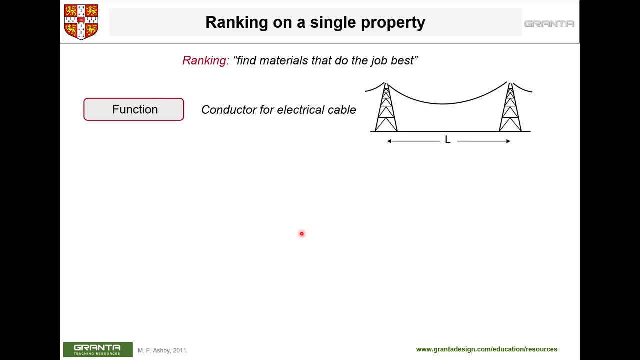 example here. let's say you want to design a conductor for electrical cable, so the length between the two pole is is fixed. you can't change that. that's out and your constraints are the length and the cross-sectional area and your design. you have to design something that won't fail under wind or ice load, so that 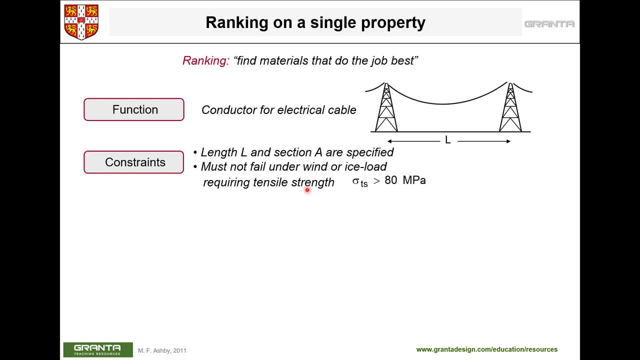 means that you're requiring a specific tensile strength. here, for example, you need 80 megapascal tensile strength for your material not to fail. the objective also is to minimize electrical resistance. if you remember, the equation for electrical resistance is Rho, which is electrical resistivity. 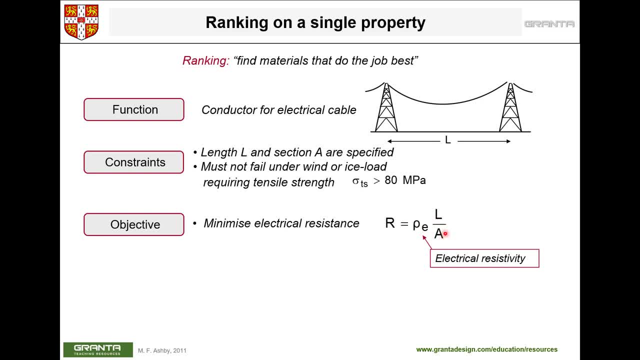 times L the length over a, which means that the longer your wire is you have more resistance, the higher the cross-section you have is in the denominator. so you have lower resistance. but you can't change L and A. you can only change electrical resistivity, which is the material property. so you could minimize this. 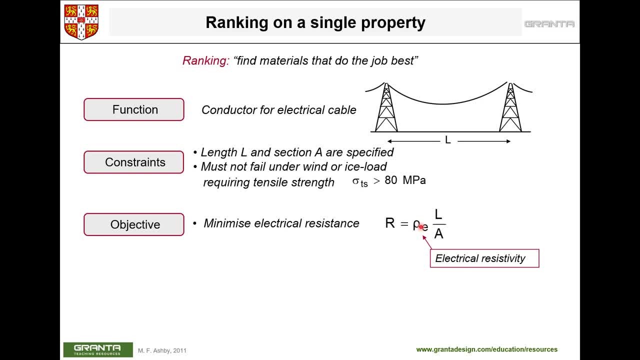 electrical resistivity and therefore your electrical resistance would be reduced. so your free variable is your material choice, because you can change the geometry. so you are gonna do a screening and select only material that are higher than have a strength higher than 80 megapascal. but you don't have any. 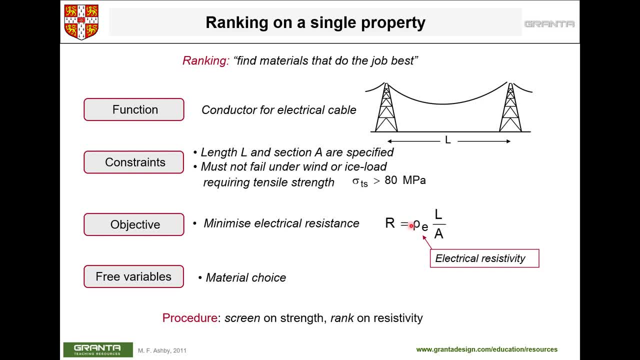 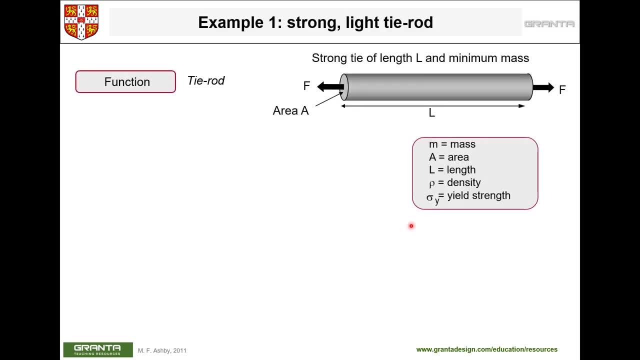 specific value for electrical resistance, so you're gonna rank them based on the electrical resistivity. let's look at another example. here we have a tie rod that is on their axial loading F and the cross-sectional rate area is A, the length is L, the mass is M. you have the specific density and 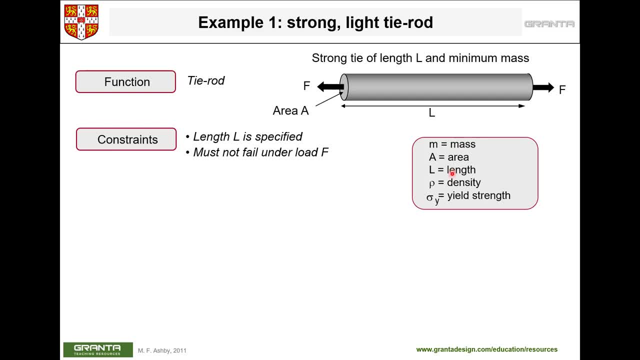 yield strength. the first three parameters are geometry parameters, the last two are material parameters. so the lengths is specified and we want, we want to make sure that our rod does not fail under load F. so we are not looking at a specific strength here, but we are looking at a specific force on that rod. 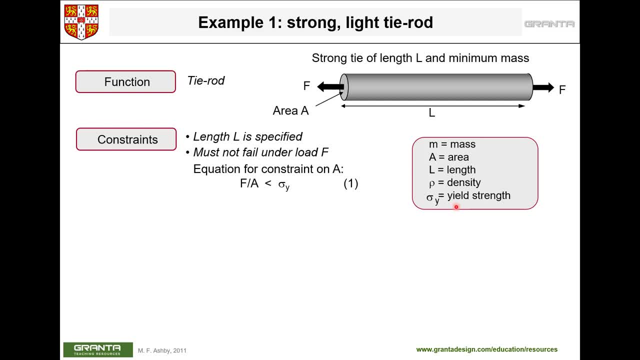 the difference here is that we have, we can, we can play with our cross-sectional area. so it doesn't matter what is the stress, as long as it doesn't doesn't fail under that particular F. so we could increase or decrease a to get our desirable parameter. also, we're going to minimize mass, so mass, the equation for 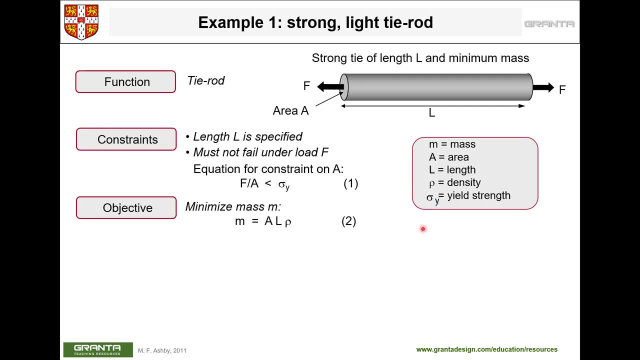 mass is density times the volume, and the volume is area and length. so you can see area appears in both terms. here for minimizing we are going to reduce a. here for minimizing because a is in denominator, we have to maximize a. so you can see we have a conflict challenge here for one of the criteria we have to 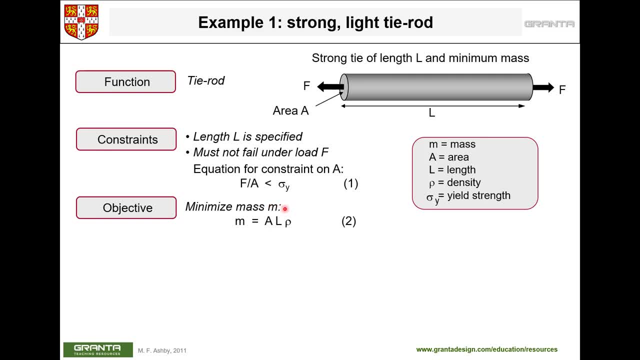 minimize a. for the other one we have to maximize a. so for that we are going to remove a from our equation and our free variable would be our material. so if I eliminate a, can write my M. that would be my performance equation function of FL Rho. 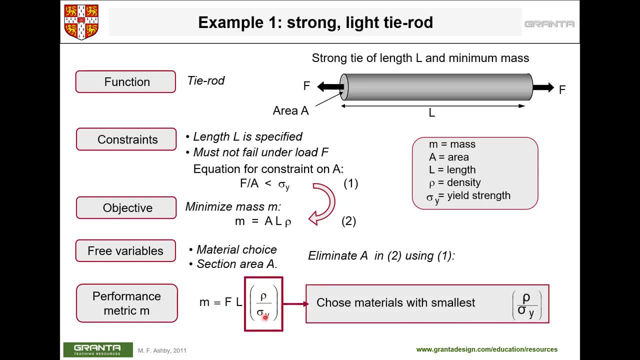 Sigma a. if I rewrite this one, you see that Rho over Sigma Y would be my material indexed and I want to minimize my material index or maximize Sigma Y over Rho. so in this equation we didn't care about elastic, modulus or other property. the material property that we care is yield strength- Sigma Y- we don't. 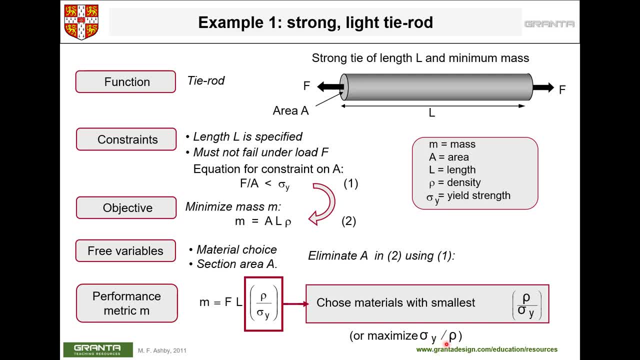 want our material to go under plastic deformation and also the density, and we have a linear equation. it's not Rho to the power of 2 or anything, it's just a simple Sigma Y over Rho. so on those plots that I show you we can go and then 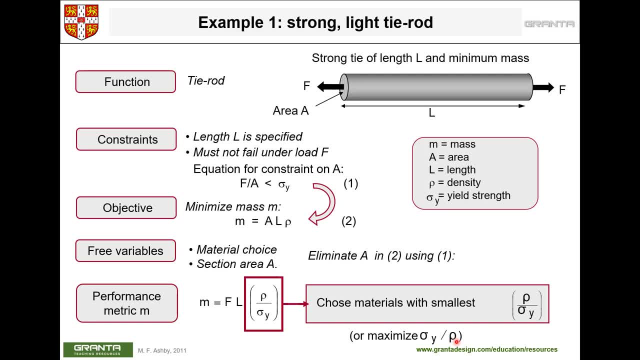 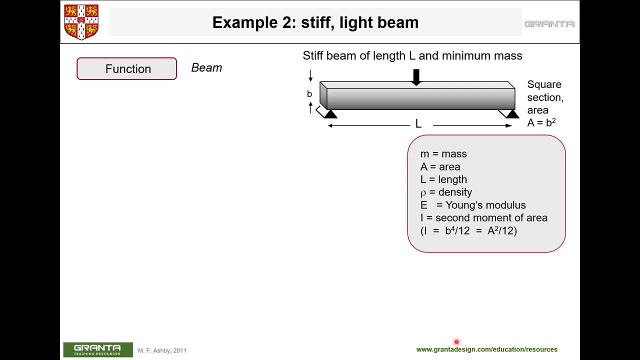 draw this line and select all the material that fall about this line. let's look at the second example here. in this example we have a beam, for the difference between beam and a rod is that the beam can have transverse deformation, so we are applying the load. 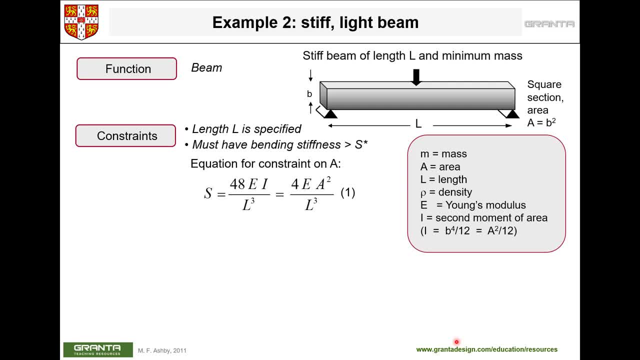 the length is L, and then we have our constraints and our objective. the constraint is that the stiffness should be higher than a specific value, because we don't want our beam to have high deflection and if you remember the stiffness of the beam or the equivalent stiffness boolean increase or decrease of 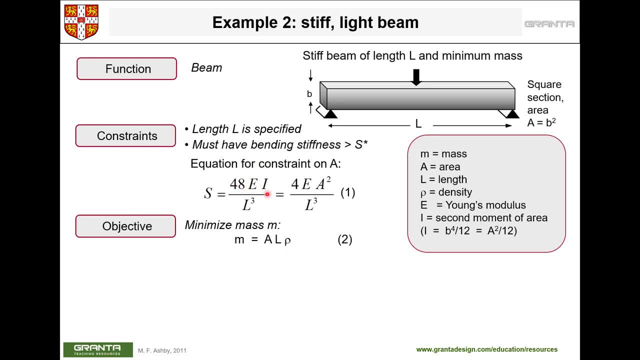 the beam is relating the force with the displacement. so that's the stiffness equation that you're gonna have, and the objective is similar to the previous problem. we're going to minimize mass, so we have area in both equation. we use the same approach. we remove the area between two equations, we eliminate it and then 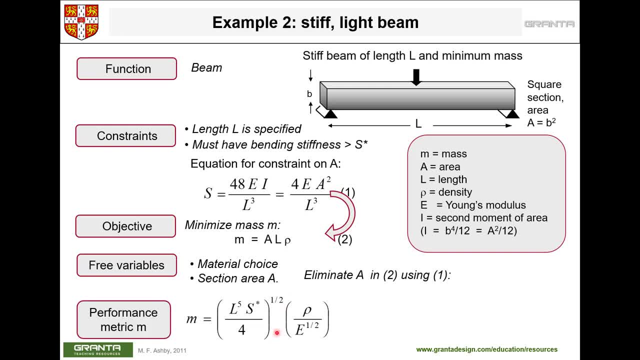 we get our performance equation. so here I have put all the geometry parameters here and then move the material, which would be our performance, in one fraction and if you want to minimize M, which means that I have to minimize this term. so here, unlike the previous equation, here we have Rho over e to the 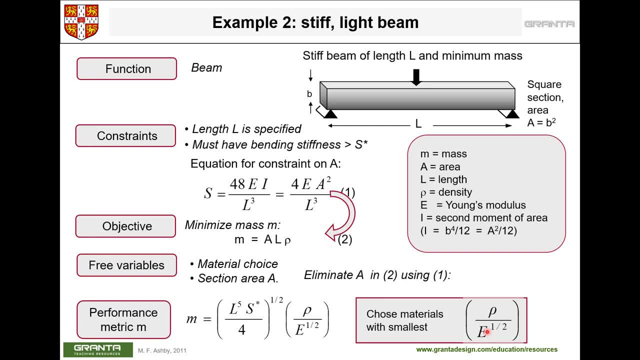 power of one to the power of half. so we don't deal with strength yield or ultimate strength, we deal with elastic modulus. so for this case we need elastic modulus. that's the property that is important for us. also, it's not a linear relationship with Rho over e to the 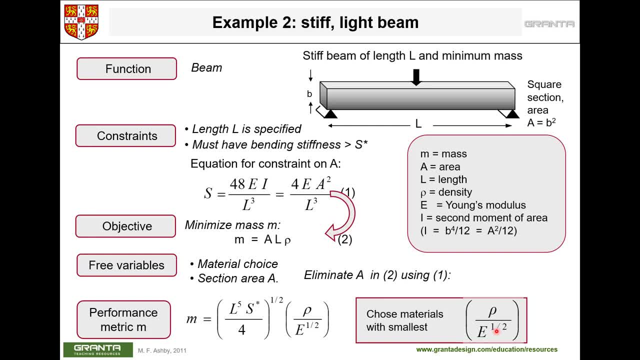 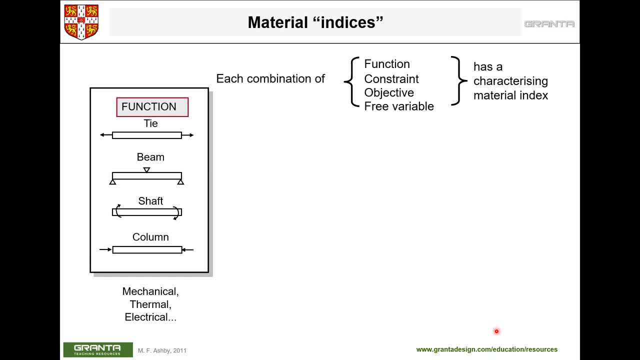 power of half. so we're going to minimize this or maximize the, the reciprocal of that. so for material indices, depending on what type of loading you have, you have a different material index. if you have a beam or a shaft or a column, your material index would be different. but the software would allow. 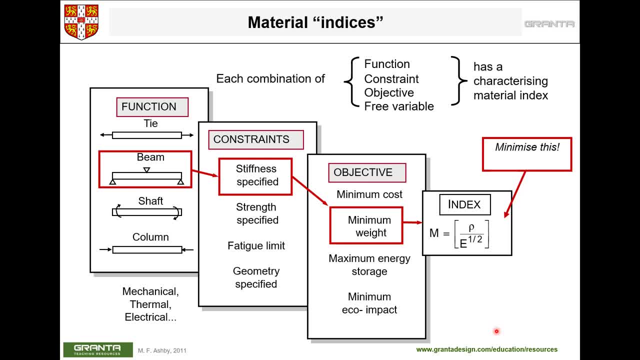 you to choose. okay, one beam I want to have. this stiffness is a constraint. I'm going to minimize weight and then that's the material index that you need to work with in minimize or maximize. finding the material index would be a task for you to look at your edge. 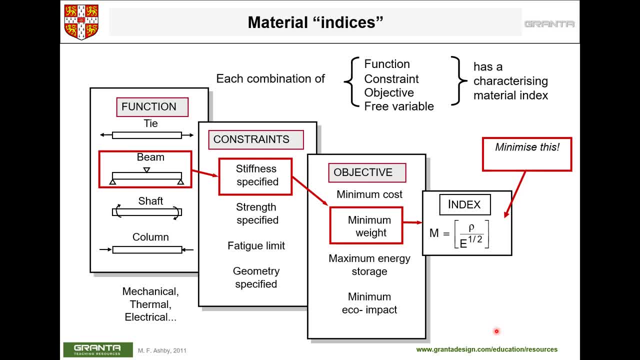 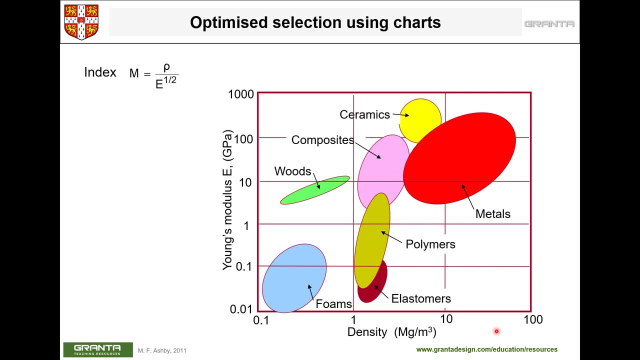 equations and find the proper material index. but for a common geometries and common loading you already have the material index here. we want to see and use the material index in our plots. so we have Rho over e to the power of half. if M- that's our constraint- that's a constant number. we said that our plots 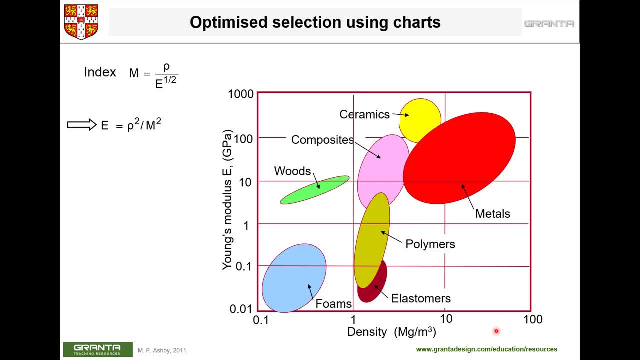 is logarithmic. so I'm going to take a, I'm going to rearrange the equation and and then take a logarithm of each side. so here, now that I took a logarithmic logarithm, pocket each side, the right and left, you can see I have a linear